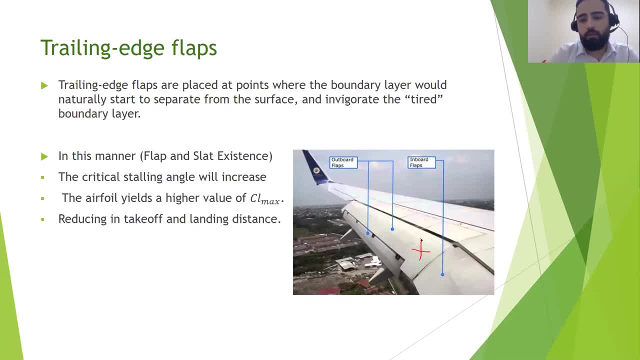 Sometimes you can find on the airplane inboard air flaps or outboard air flaps, And this one, its name is ailerons. The trailing edge flaps are placed at points where the boundary layer would naturally start to separate from the surface. 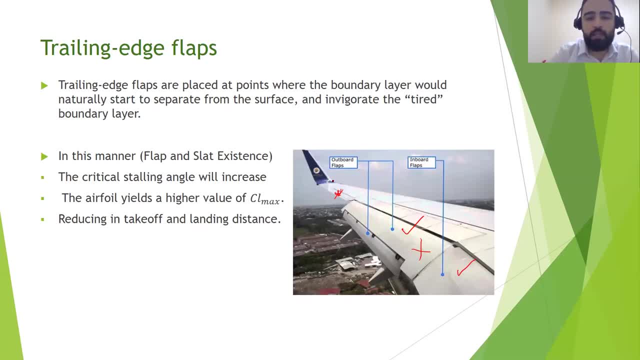 And invigorate the trailed boundary. So The airfoil has a boundary layer. So here we have a boundary layer. At the upper surface, At this point we have tired boundary layer. So the location of the flap, of the flap, Ensure to strong or to invigorate the tired boundary layer. 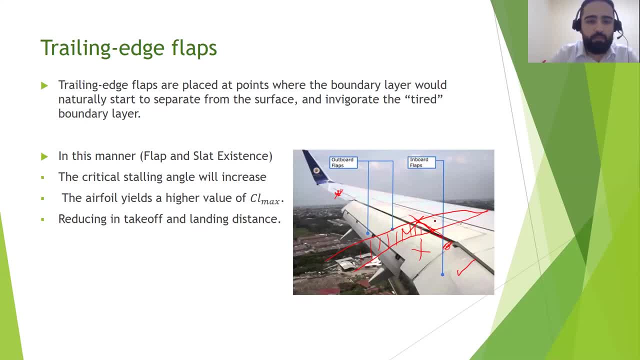 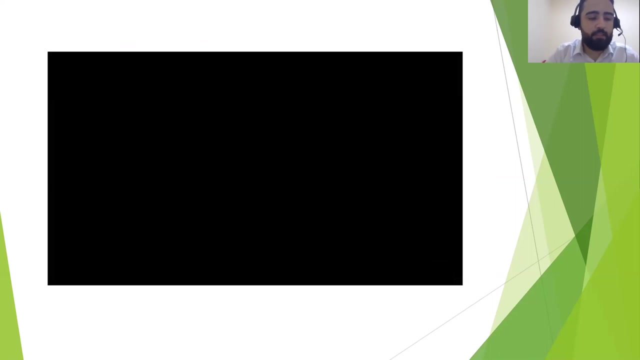 So In the airplane, If we have a flap and the slot at the same time, what will happen? the critical stalling angle will increase the airfoil yields a higher CL max value of CL max, reducing intake of and landing distance. I will show you a video before I continue this. 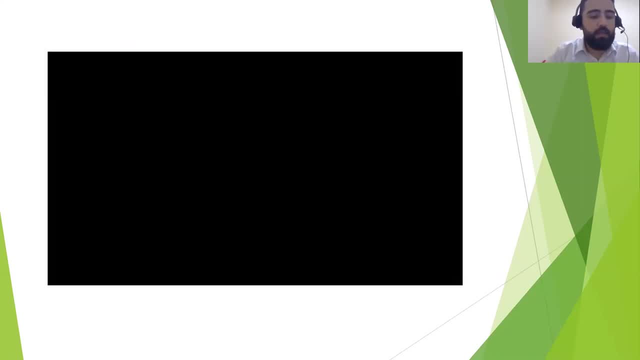 video contains the following topics. this video talk about the trailing edge flaps, relation with the angle of attack, some types of the flap, like a plane flaps, splitted flaps, etc. and what will happen for the CL versus angle of attack graph with flaps if it's an up position or in. 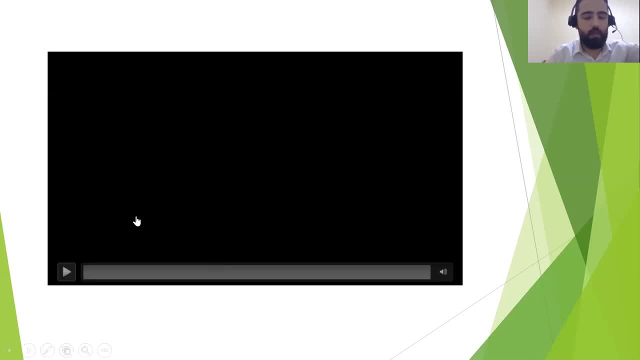 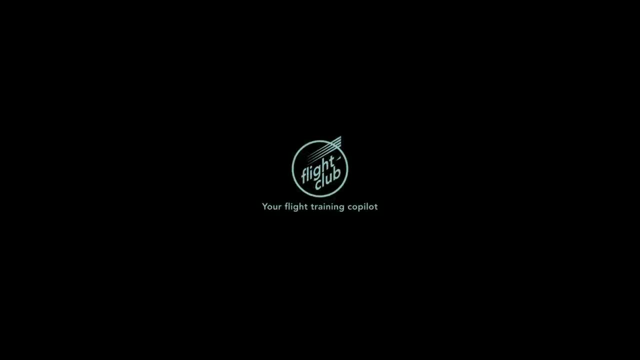 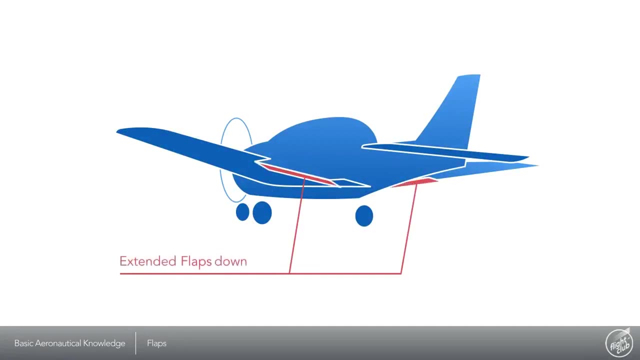 down position. I will leave you with this video and I will come back to you. flaps are secondary control surfaces mounted on the trailing edge of the wings. they are primarily used to accommodate safe, slow flight and to shorten the takeoff and landing distances on the ground. there are 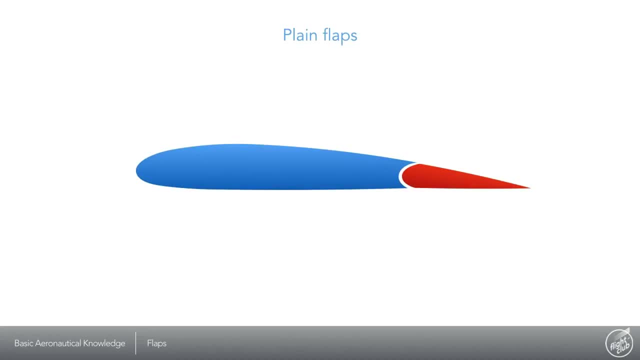 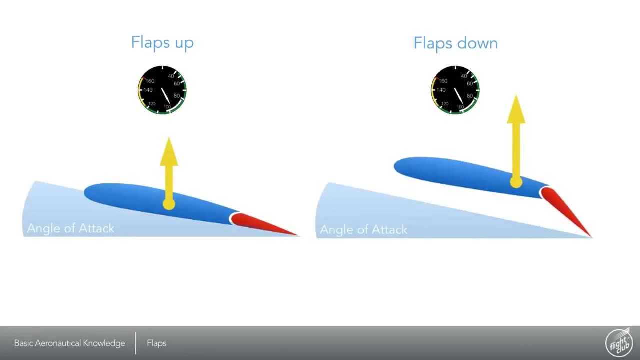 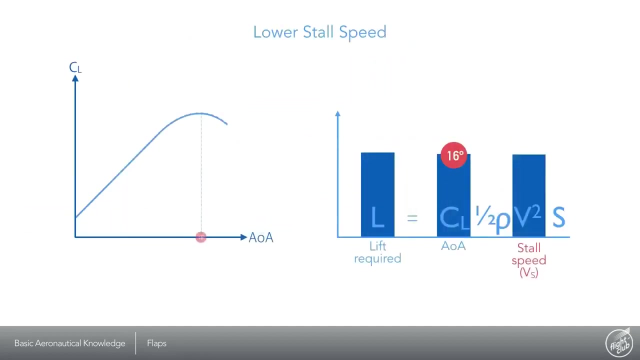 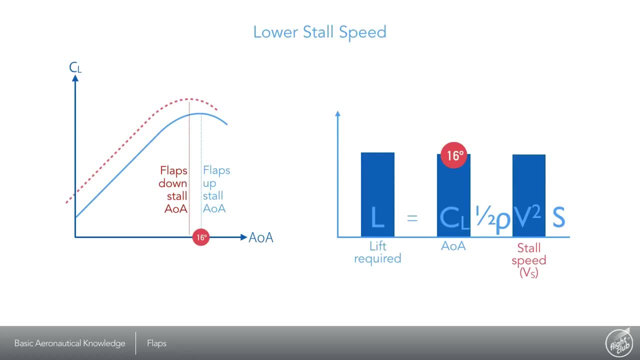 down. According to the lift formula, greater ability to generate lift translates to a lower stall speed. once the stall angle of attack has been reached, The flaps down configuration assumes an effective angle of attack that is relatively larger than the actual flaps up angle of attack. So the aeroplane will stall at a lower nose attitude with flaps. 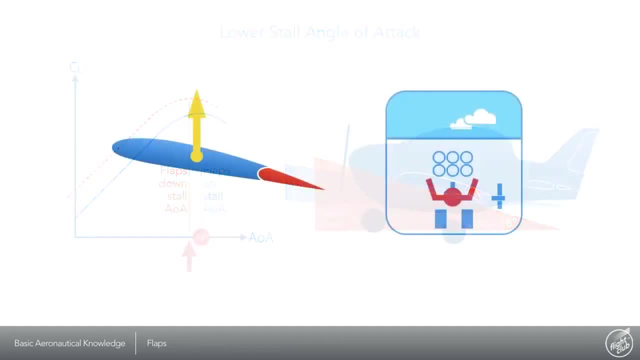 down compared with flaps up. With flaps down, the aircraft is able to maintain lift at lower nose attitude. This means that the pilot gets improved visibility down below, which is especially handy when landing. Some other flaps designs found on light aircraft are split flaps. These 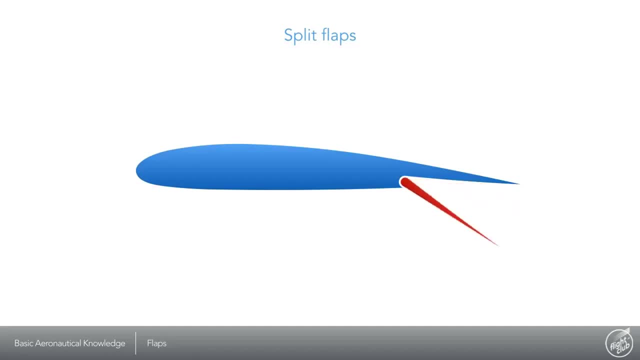 are hinged below the wings. Subtitles by the Amaraorg community. When extended they increase lift but also cause a lot of drag when compared to the plane flap design. The drag is due to the extra disturbance of the airflow around the wings. 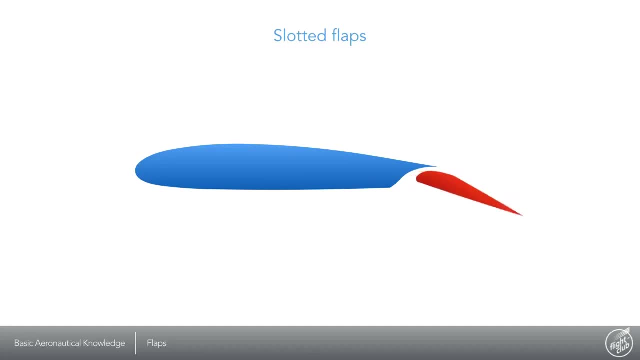 Slotted flaps are similar to plane flaps, except for a slot that allows the higher air pressure below the wings to flow up through to the lower air pressure above. This helps the airflow remain attached to the flap, thus increasing lift. Flaps are similar to slotted flaps but they move back and down. when extended, They increase. 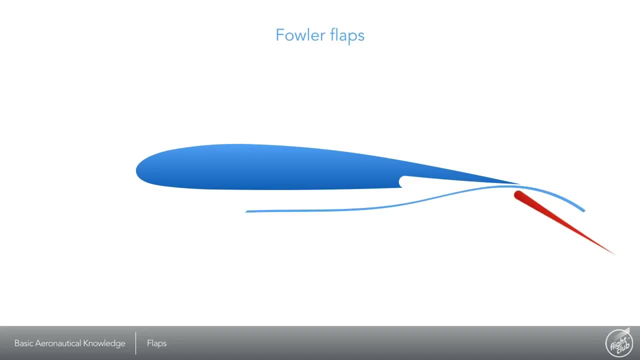 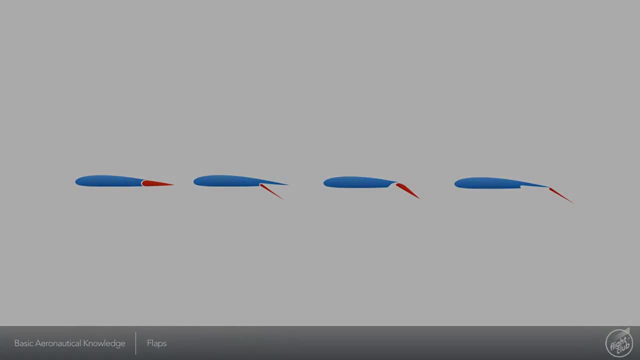 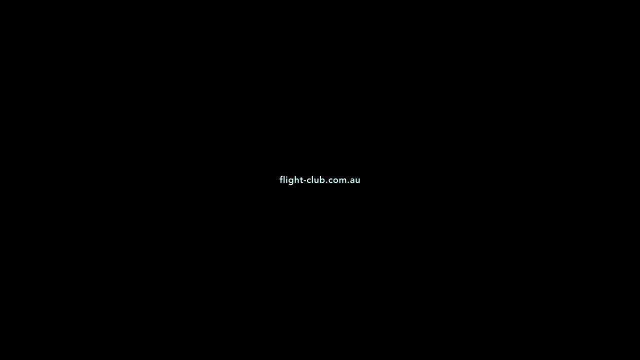 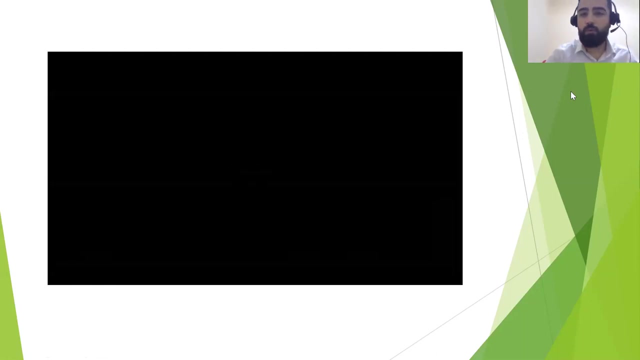 the effect, with wing surface area and camber resulting in more lift. Of course, there are more complex flaps designs found on larger aircraft, but we'll look at those another time. I think after watching this video- or I am sure that now all of you want to know more- 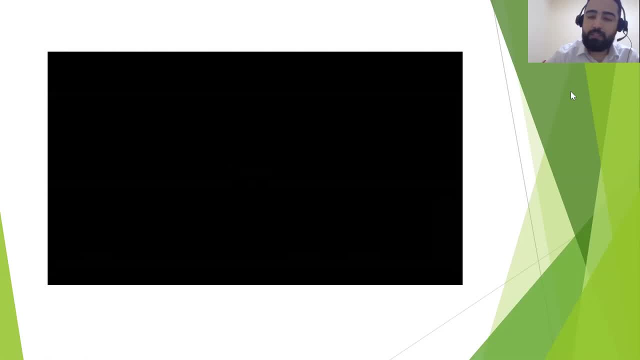 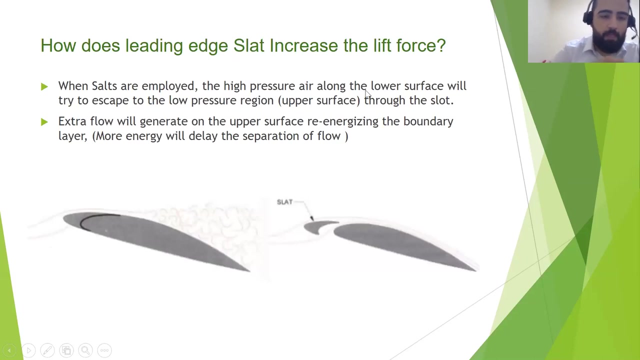 have these questions in your mind: how does the leading edge slat increase the lift force? or we have another question: how does the trailing edge flap increase the lift force? okay, let us talk about this and this slide. here we have the airfoil. this is a cross section of the wing, this is the leading edge slat, and 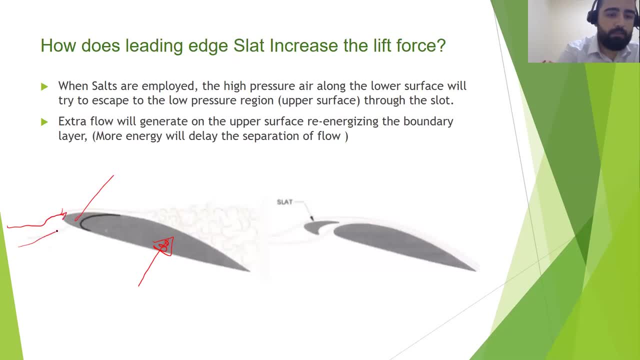 the flow come from this side and it will cover the upper and the lower surfaces. at the upper surface, after a specific distance or a certain distance, the boundary layer will be very weak and you you Look at these patterns of air flow. that means the flow separated from the surface. 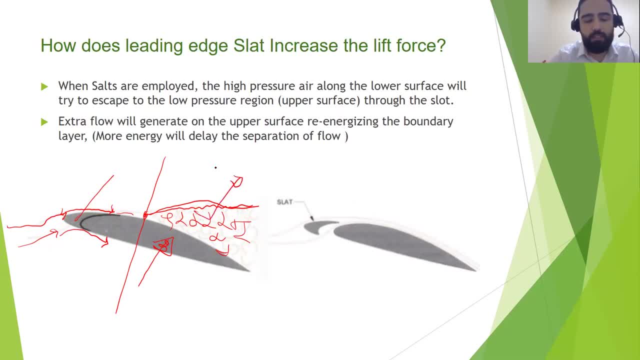 Okay, this is called separation drag or form drag. Now what will happen if we add this part on the wing? This is the slot. you can move it forward, generating this gap, the slot. Here in this area we have a high pressure region. 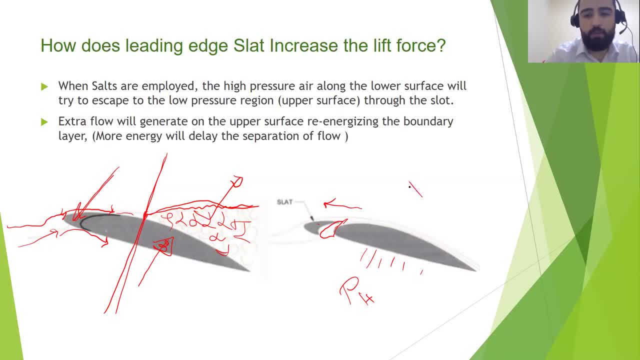 And in this, in the upper surface, we have low pressure region. The resultant of the high and the low pressure will make the lift force And, as the nature of the materials, if we have two regions- high pressure and low pressure- the nature of the material. it will make it to move from the higher pressure zone to the lower pressure. 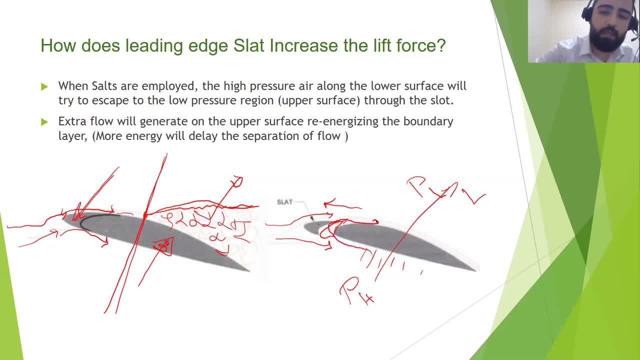 so that the air flow will come from this gap, from the upper surface to the lower surface, like this. Okay, let us read these sentences. The first one: when slats are employed, the high pressure air along the lower surface will try to escape to the low pressure region. 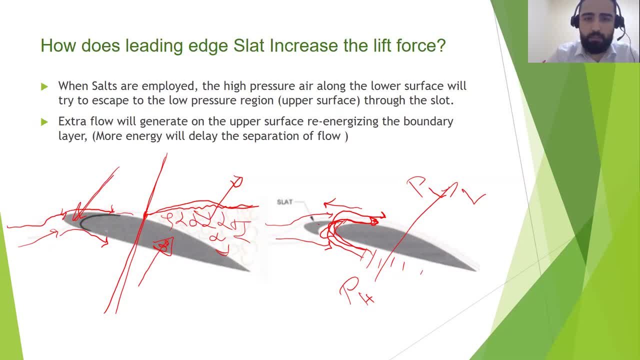 which is this upper-lower region, is the upper surface. through the slot, Extra flow will generate on the upper surface come from the lower surface. this extra flow re-energizing the boundary layer, That means this area or this side of the boundary layer, will re-energize. 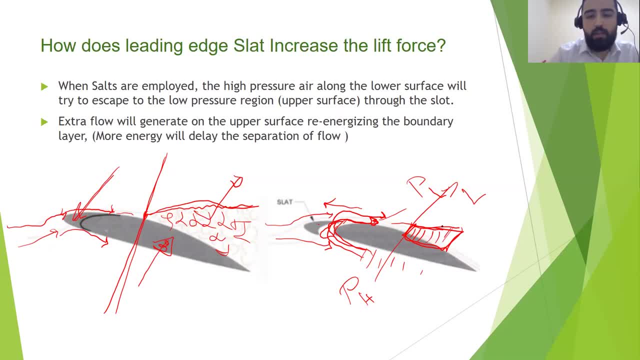 That means more energy. If it has more energy, or if we have more energy in this region, that means the separation flow will be delayed. Instead of starting from this point, it will start, for example, from this point. What about the trailing edge? 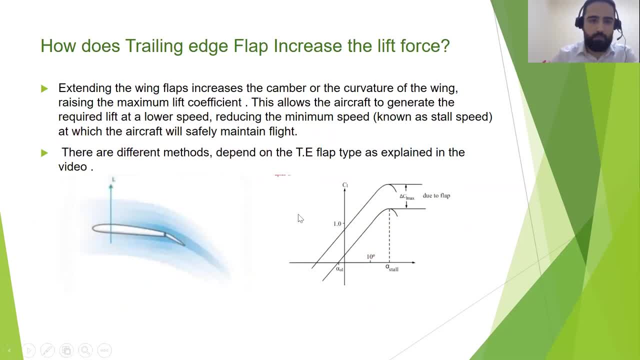 Flap. Extending the wing flaps increases the camber or the curvature of the wing, rising the maximum lift coefficient. This allows the aircraft to generate the required lift at lower speed, reducing the minimum speed, known as stall speed, at which the aircraft will safely maintain flight. 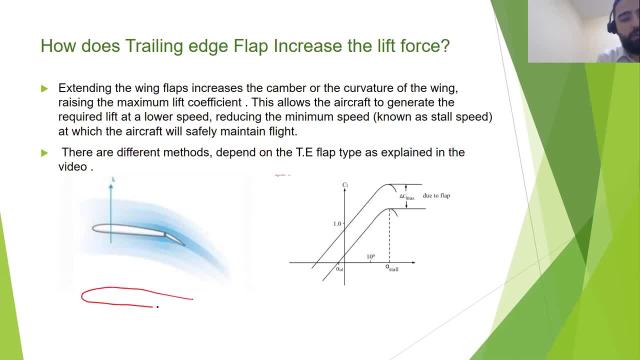 We have the original flap or the original airfoil. It was like this and we have here extended flap. Once we deploy the flap, the cord line was like this, and now this is the cord line. First of all, we increase if the relative flow in this direction. 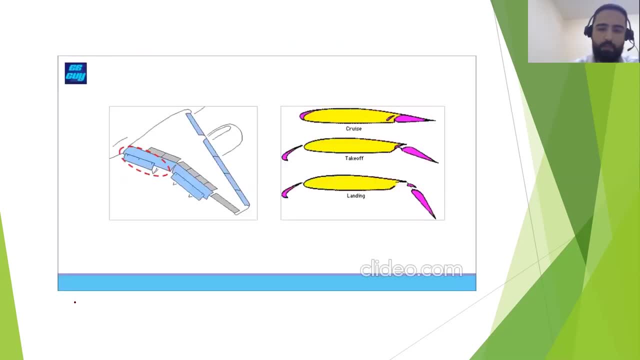 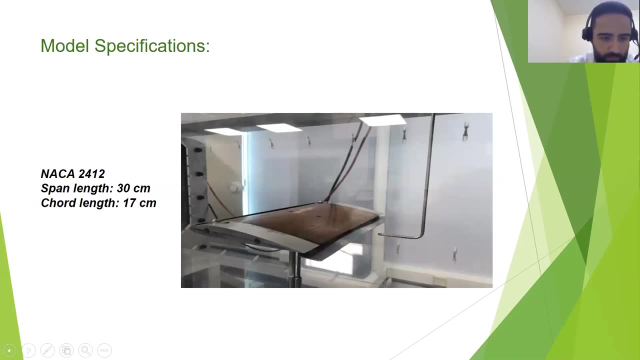 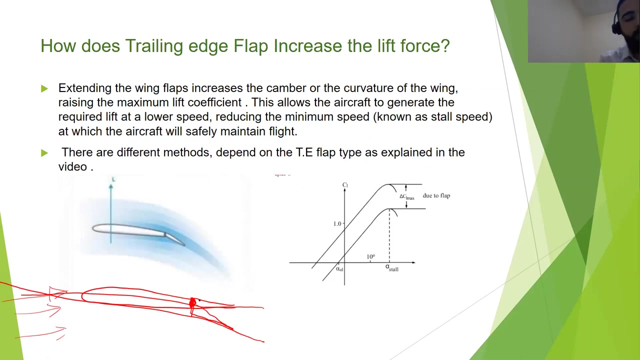 so we increase, sorry, we increase first of all the angle of attack, because the angle of attack definition is the angle between the cord line and the relative flow. And the second thing: we increase the camber line. The camber line was like this: 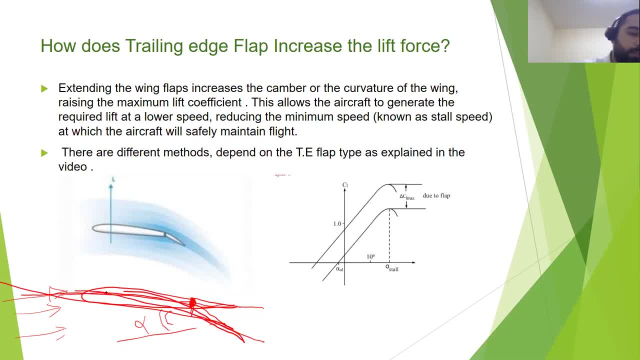 and now it's like this: So more curvature in the wing. These two specifications gives the airfoil the ability to introduce more lift or to increase the maximum lift coefficient. There are different methods. there are different methods depend on the trailing edge flap type. 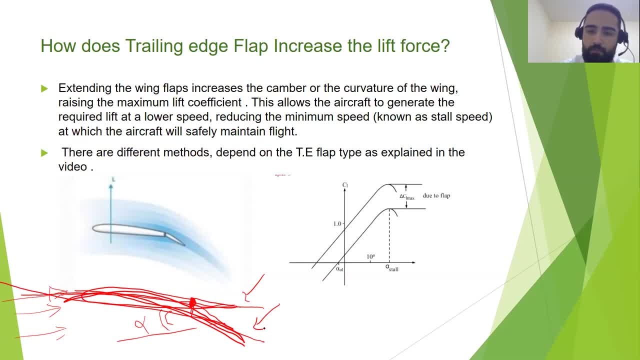 as explained in the previous video. If we look to this graph, we will see that this is the original flap and this is the flap. this is the original airfoil and this is the airfoil. due to flap angle change, You will find that in the plane flap. 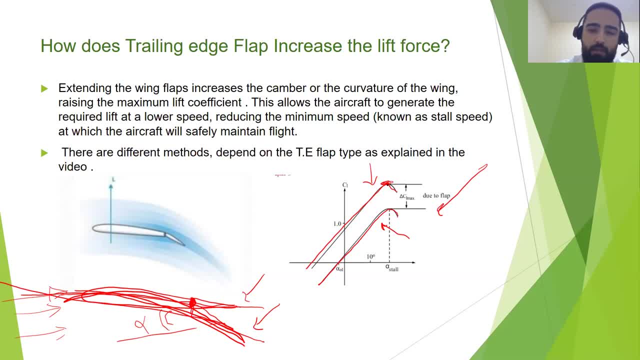 C L max will increase but the alpha stall will decrease. But in another type of flap they can increase both of them: C L max will increase and alpha stall will increase. For example, split airfoil can make this graph similar to this one. 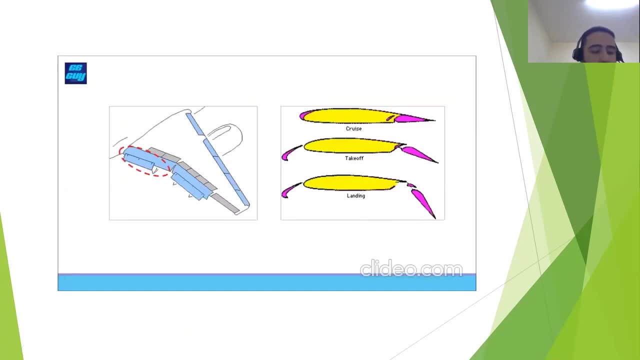 Now this video contains the flap and the slat position, or the effect of the flap and the slat position during the landing, takeoff and cruise segment in the flight. So let us also watch this video and I will come back to you again. 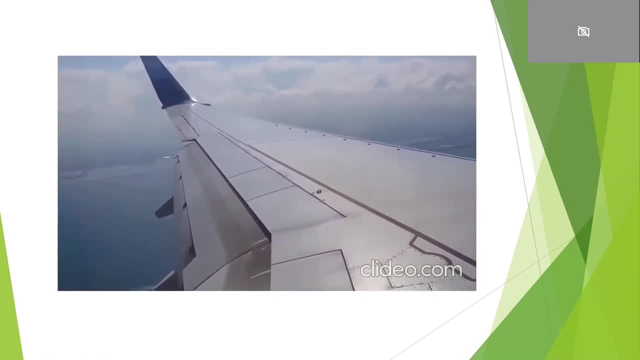 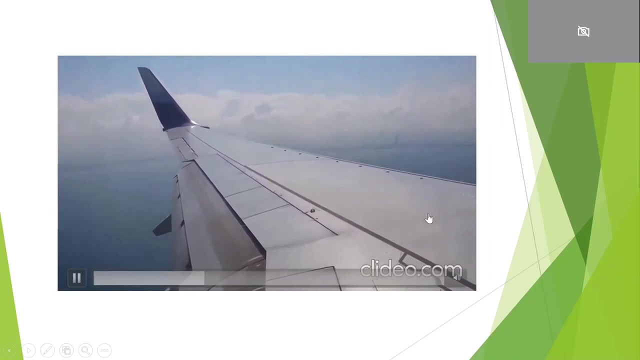 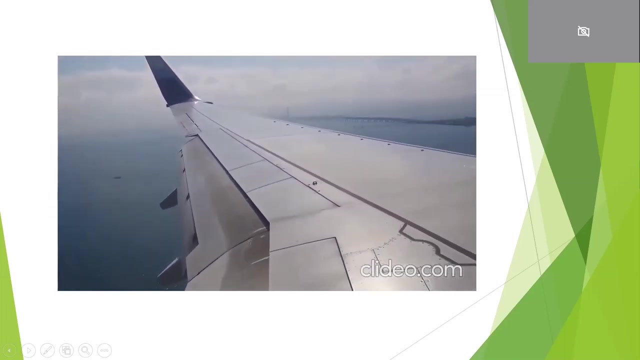 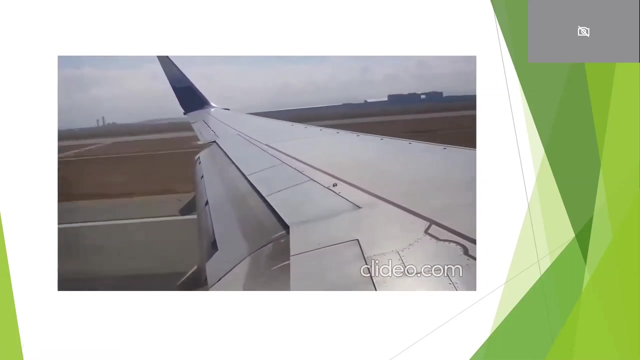 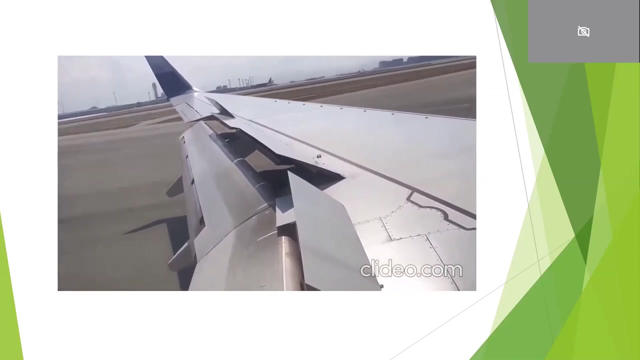 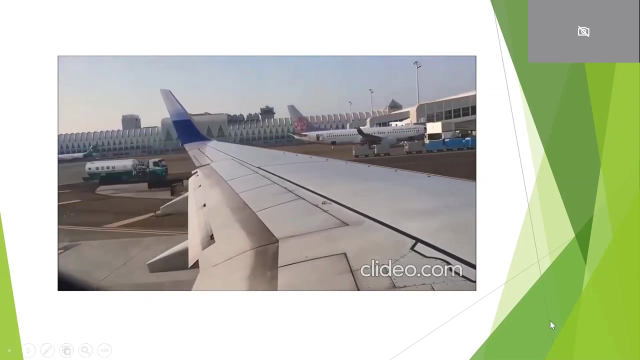 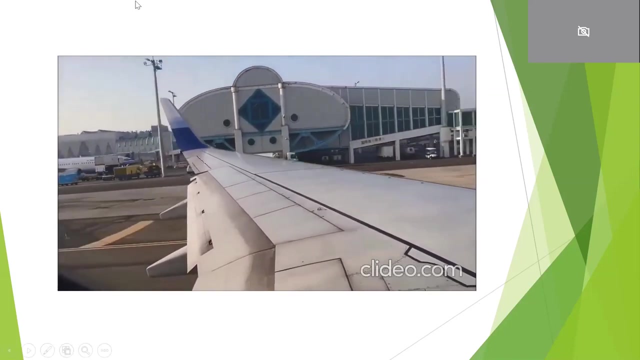 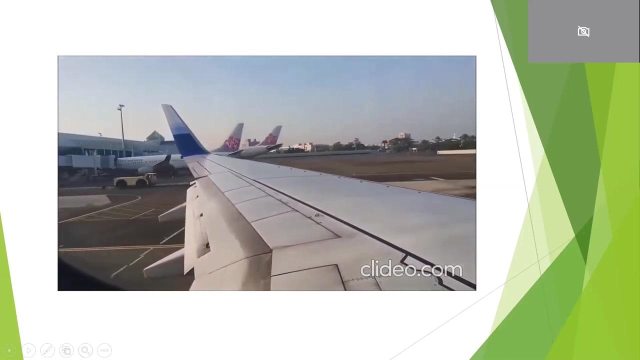 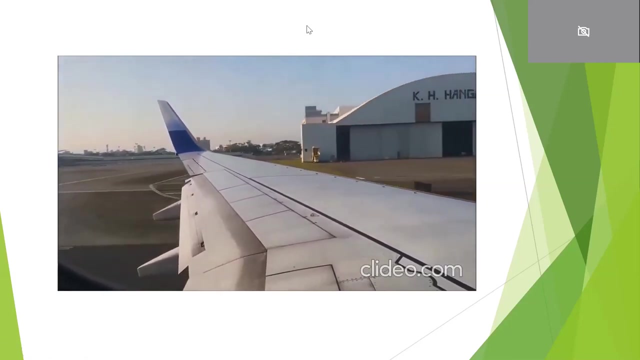 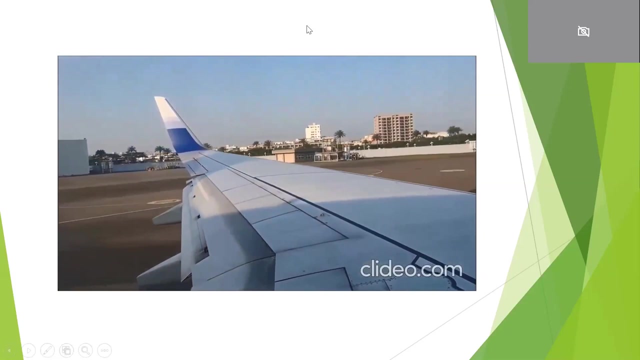 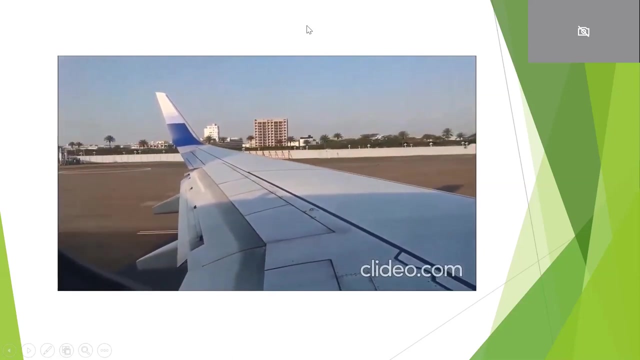 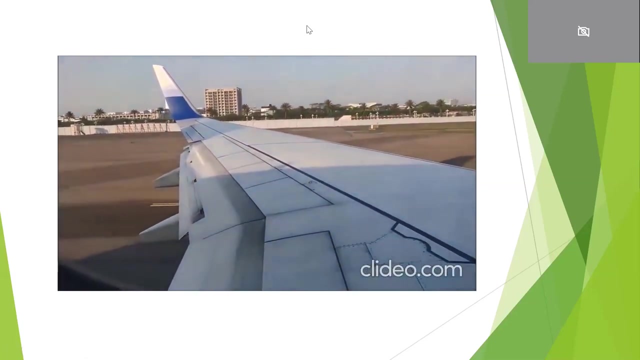 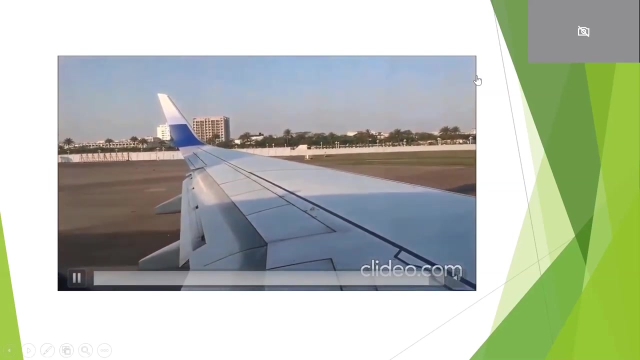 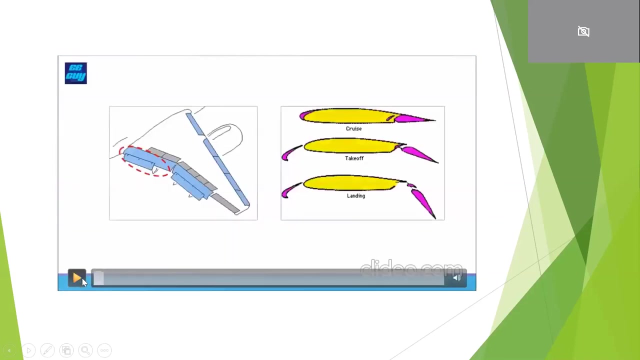 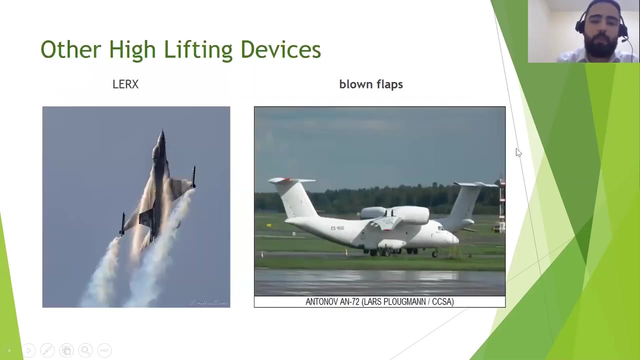 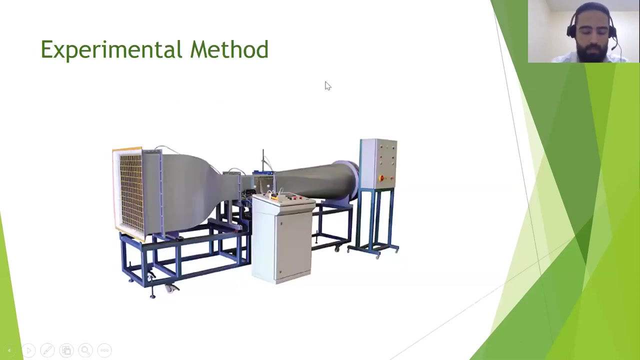 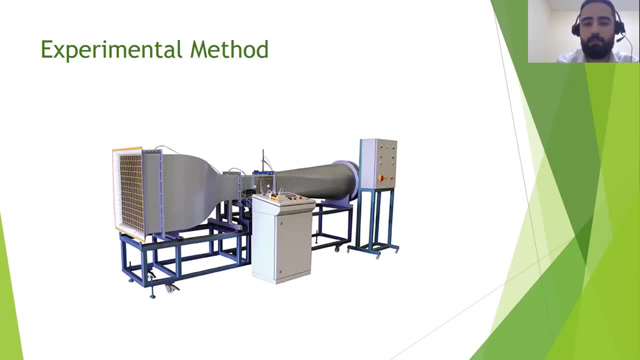 Now let us talk about the experimental part, or the experimental method in this lab. This is the subsonic low-speed open circuit wind tunnel. We used this wind tunnel before in this course, As we know. this is the variable frequency drive control unit. 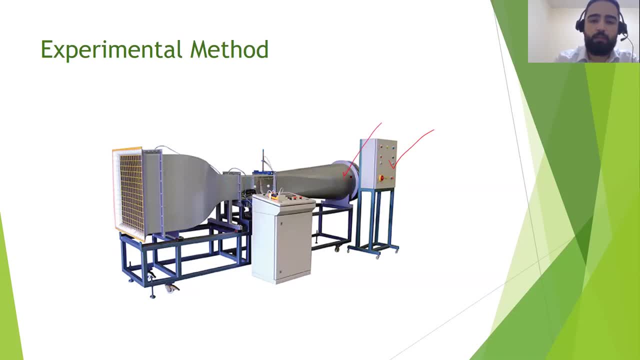 To control the speed of the motor: the motor inside this part. this is the convergent part and this is the divergent or contraction cone. We have the test section and here the control unit. From the control unit, this one, we can measure the speed inside the test section. 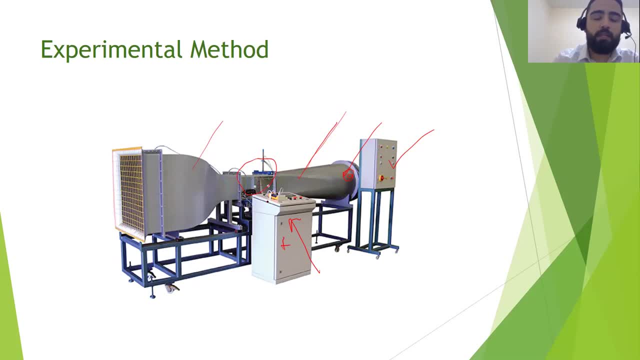 and we can measure the load cell, The load cell existing here Under the test section. this load cell read the lift and the drag and the moment from the models and transfer these signals to the control unit and we can read this value on this display. 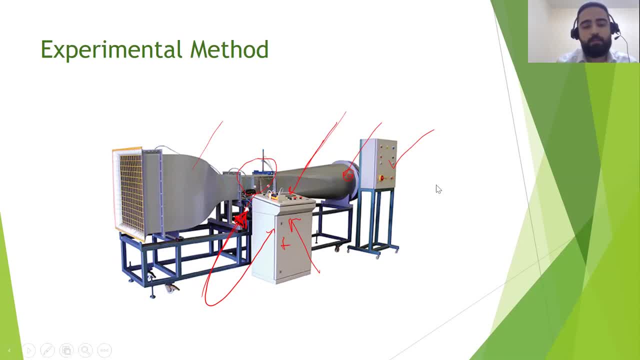 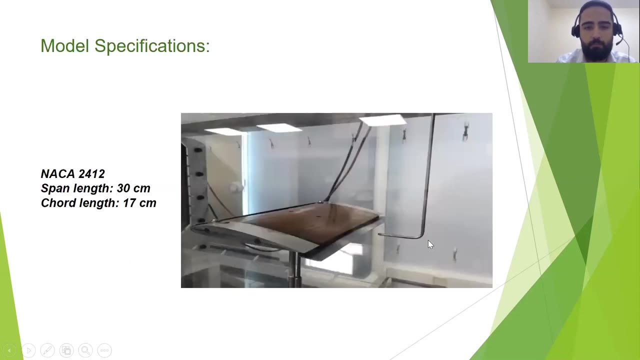 Okay, So we will use the imagine that We will use this wind tunnel and we will insert a wing model inside this test section to take lift, drag and moment data. This is the wing We have this wing. The wing family is NASA 2412, as you see here. 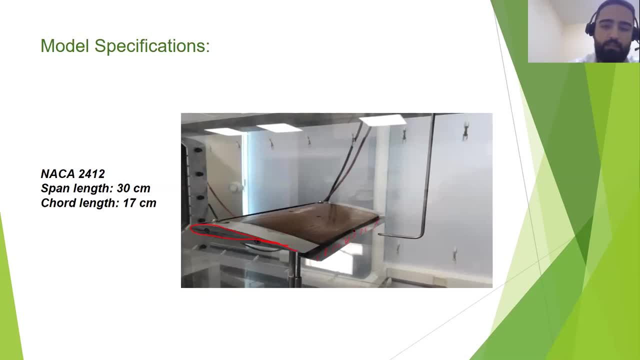 Here we have trailing edge flap And we can adjust its angle, like this, for example, or like this. We have also here slat. We can open it to make a gap between the slat and the airfoil itself, or we can close it to make it as one part with the airfoil or with the wing body. 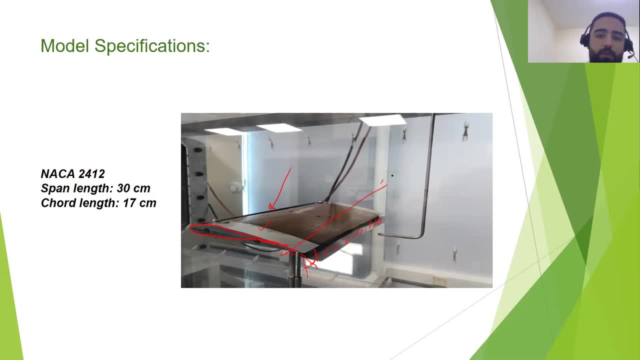 The span length of this airfoil equals 30. Centimeter and the cord length of this airfoil equal 17 centimeter. We will put this wing inside the previous wind tunnel. We can change the angle of attack from this stock and we can change the angle of the flap. 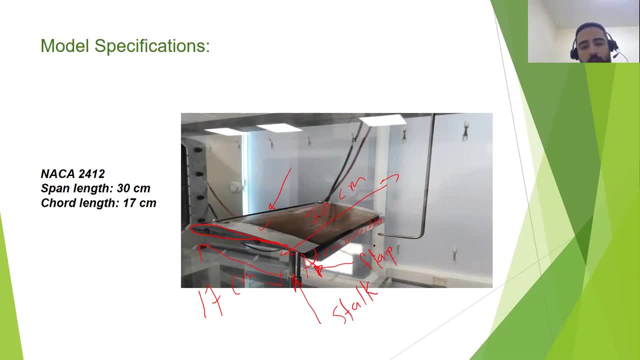 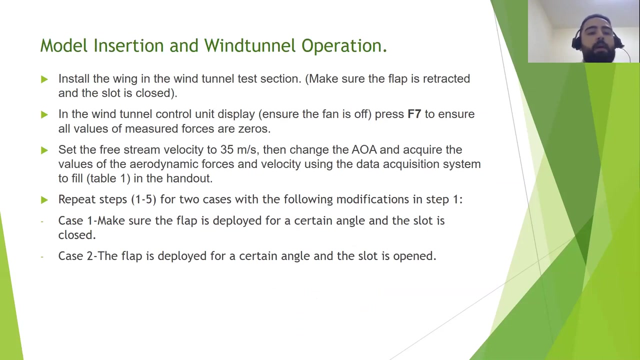 or flap angle. Okay, So here we can change two types of angle: The angle of attack from the stock and the flap angle manually, by hand to this airfoil. Okay, Now let me concise the procedures: Install model insertion and wind tunnel operation. 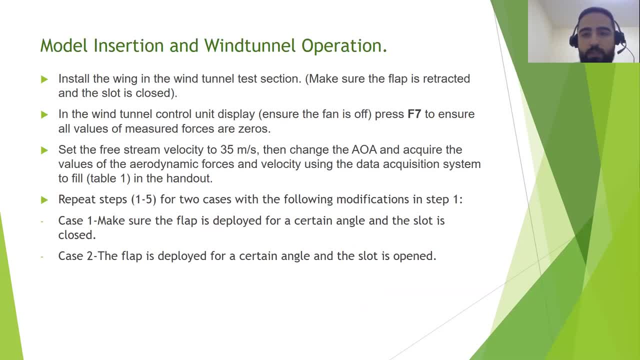 Install the wing In the wind tunnel test section. make sure the flap is retracted and the slot is closed. This is the first case In the wind tunnel control unit display: ensure the fan is off. Press F7 to ensure all values of the measured forces are zero. 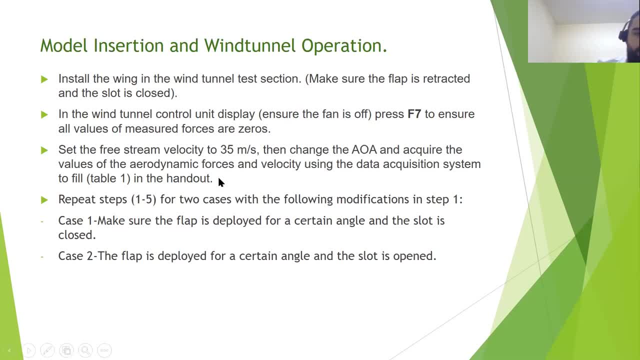 Like what we did before in the in lab number three and four, Set the free stream velocity to zero. Set the free stream velocity to 35 meter per second. Then change the angle of attack. Change the angle of attack and acquire the values of the aerodynamic forces and velocity using data acquisition system to fill the table number one in the handout. 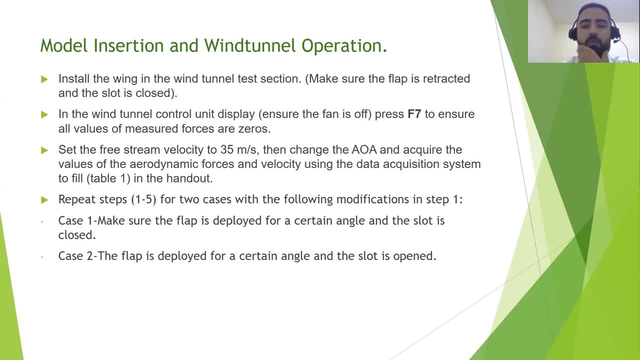 So I think we have sent for you a handout. You can find it on the blackboard system Hand out. It's for lab number six. You will find table number one to fill it with the recorded data. Repeat the step from one to five for two cases, with the following modification in step one: 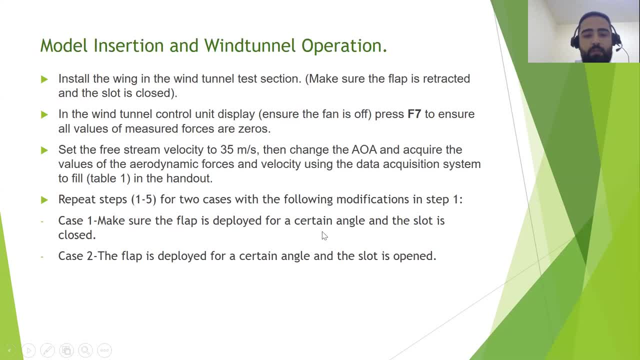 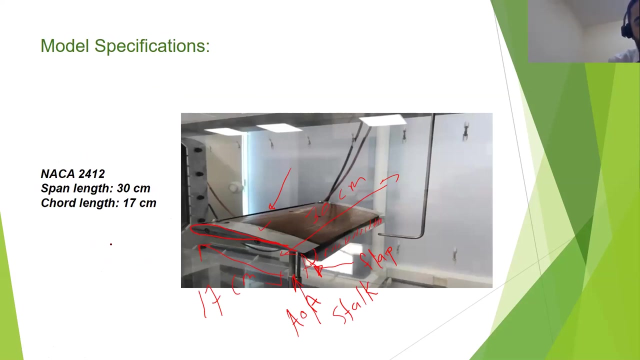 Case one: Make sure the flap is developed for a certain angle and the slot is closed. Case two: The flap is deployed For a certain angle and the slot is opened. So now, after finish this step, we have three cases. Let me show you the first case. the first case. 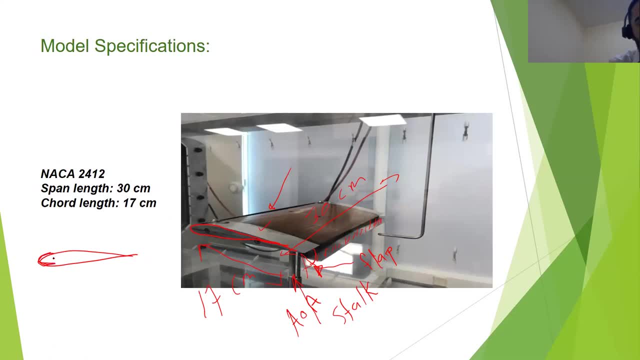 Flap with a closed slot and with extended flap. Case number two: Close the slot. No slot with, For example, 23 angle of a flap degree. this is degree okay. and the third case: at the same angle of a flap 23,. open the slot. 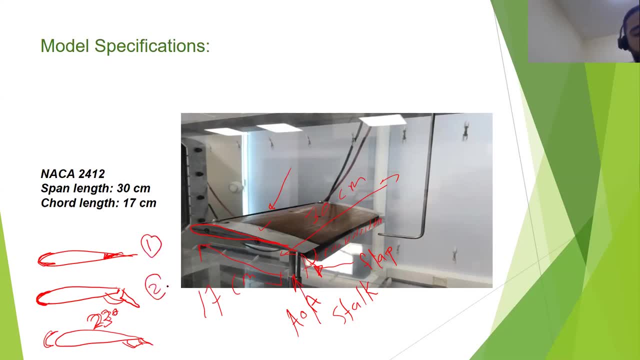 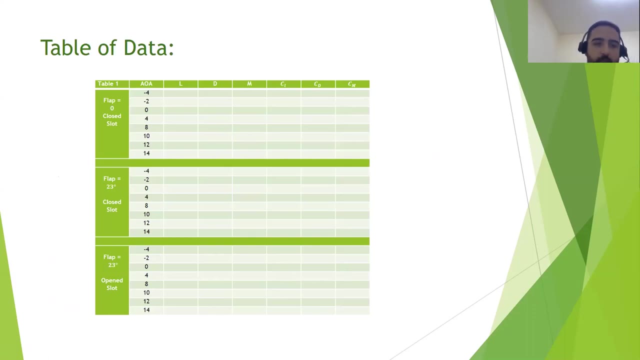 So we have this case number one, this case number two and this case number three. okay, Okay, Now we will fill in this table. Put in: this is the case name. flap equals zero. close the slot and record the data from the load cell. lift, drag and moment. 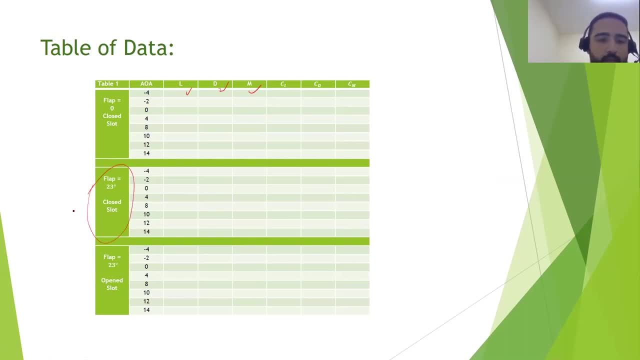 In the next case, flap 23, and close the slot. again a different angle of attack. fill in, lift, drag and moment. And this is the third case- a different angle of attack. After you fill this table, you finished the experimental procedure. 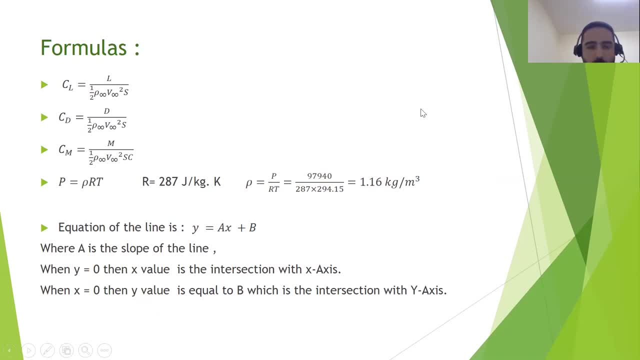 Now let us talk about the theoretical, or what you should do in this report. You should use these formulas: CL, CD, CM for finite wing, The gas law, To measure the density. but we here we have calculated the density already, which is equal to 1.16.. 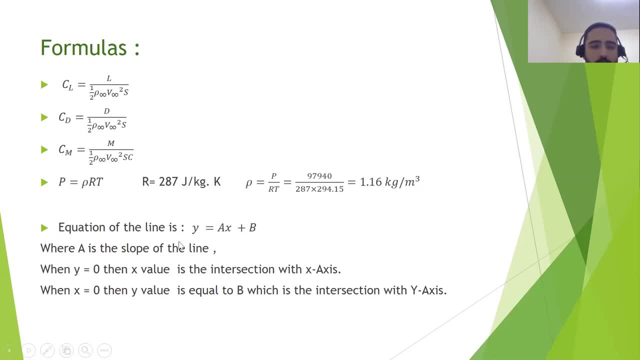 And you have to read these laws. equation of the lines is: y equal a, x plus b, where a is the slope of the line when y equals zero. So now, x value is the intersection with the x axis, So x equal. 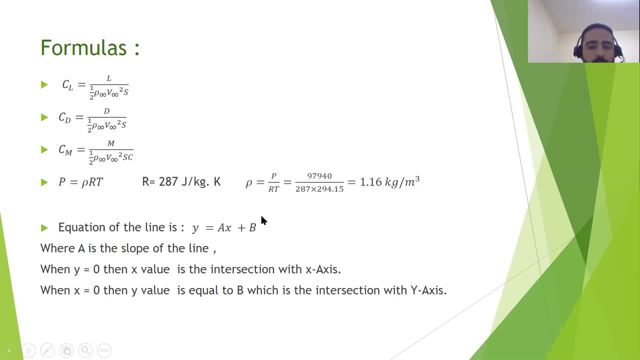 Minus b over a, which is the intersection with the x axis. When the x equals zero, then y value is equal to b, which is the intersection with the y axis. For example, this is: We have a line here. The equation of the line equal y a, b, y, x plus b. 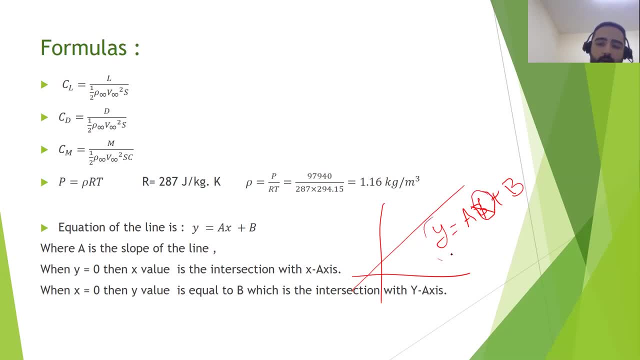 x, Y A B. The slope of the line a. Okay, The intersection with the y axis b. The intersection with the x axis: equal. When y equals zero. that means x equal Minus b over a. 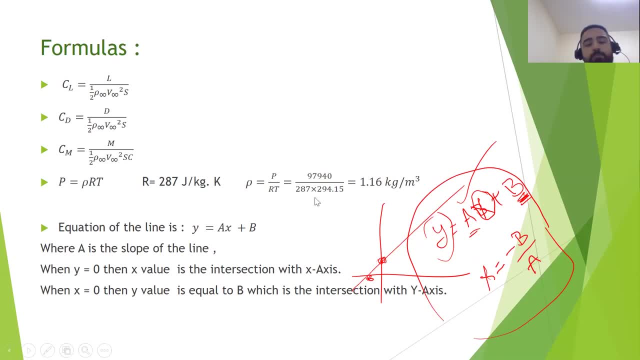 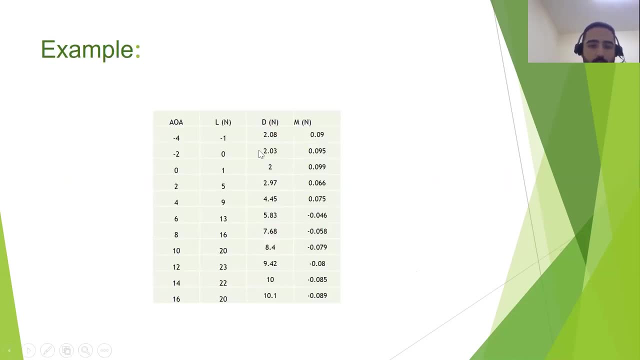 You should know these equations for the linear line To. So, For Completing this report, Okay, here I will show you a simple example: fake data, How to deal with this data, and after that You will find another data in the handout. 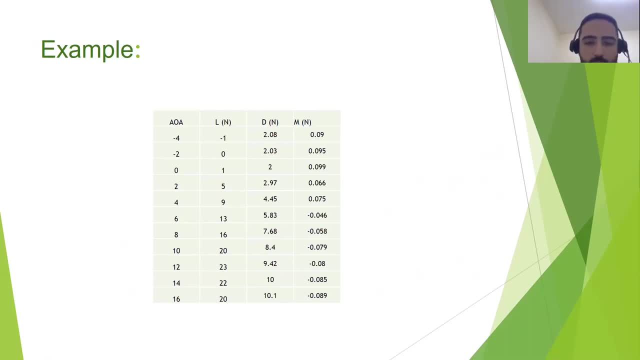 You have to make the similar procedure, What I will do now. So imagine that We have a wing and we change the angle of attack from minus 4 to 16 and we increase the angle of attack in increment of 2 degree. after that we record the lift, drag and the moment. 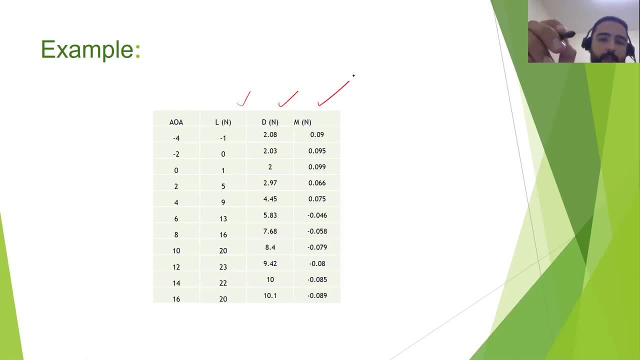 from the load cell. you have this table in the handout. you have it already with its data because, due to this circumstances of COVID pandemic, we cannot go to the college and take this reading or data. so we will provide you by this data and you have to only deal with. 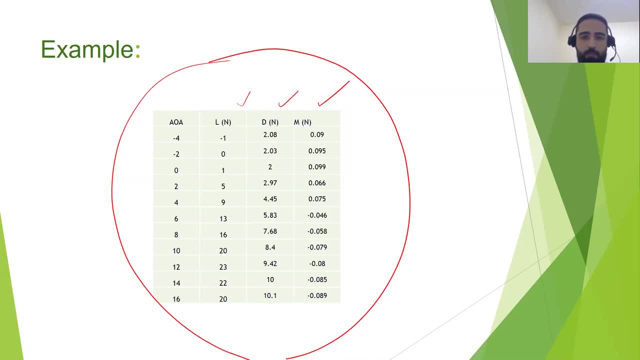 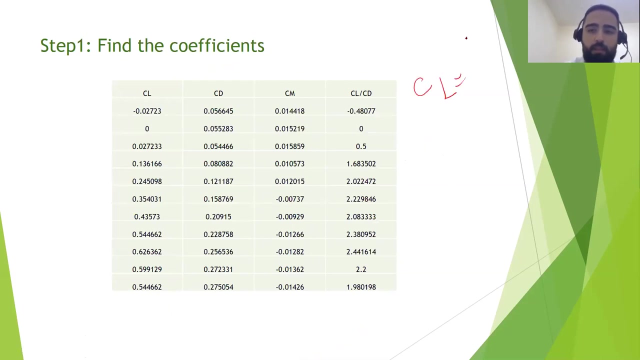 play with this data and give us the final results. ok, what should we do now? the next step? we should find CL capital, CD capital, CM capital using the previous formulas. so, for example, CL equal the lift over half rho V square Vs, where S: 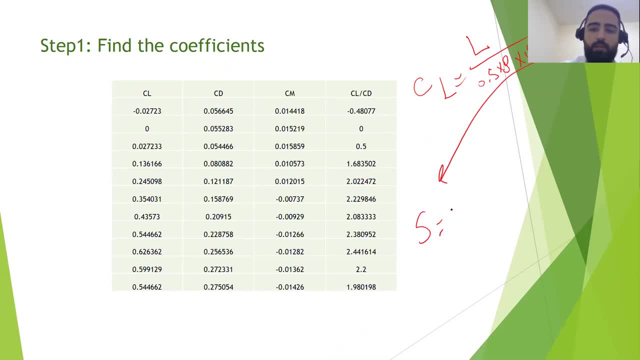 equal 0.17 multiplied by 0.17, multiplied by 0.3, because these are dimensions of our wing. so, and we have the lift in the previous table, rho, we measured this already- equal 1.16. the velocity is. imagine the velocity here. 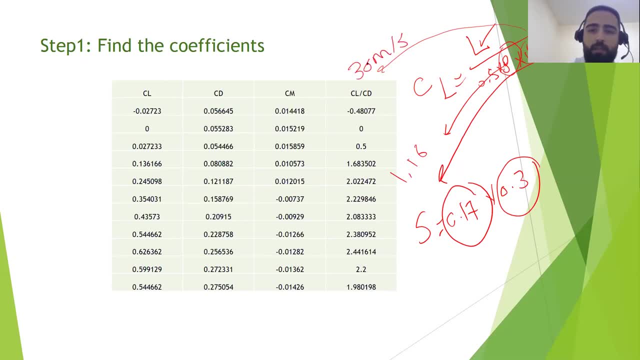 equal to 30 meter per second, but in the handout I will assume that the velocity of the wind tunnel equals 35 meter per second. from this equation we can find this number. when you drag and drop, you will find everything. just program the first cell and you can find the others. 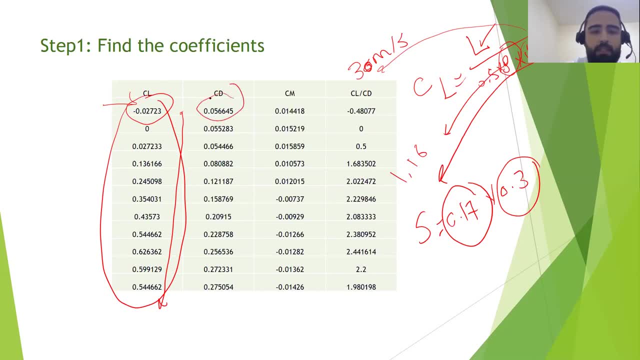 in a similar way we have another formula for the first CD and using the excel, drag the first cell to measure the other cells and for the cm s multiplied by c. for cm, cm, equal moment half multiplied by rho, multiplied by v square multiplied by s multiplied by c. 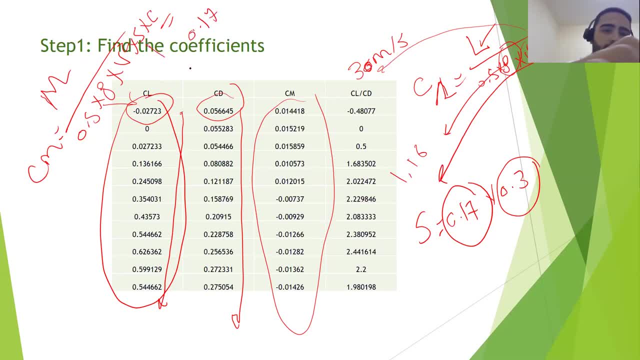 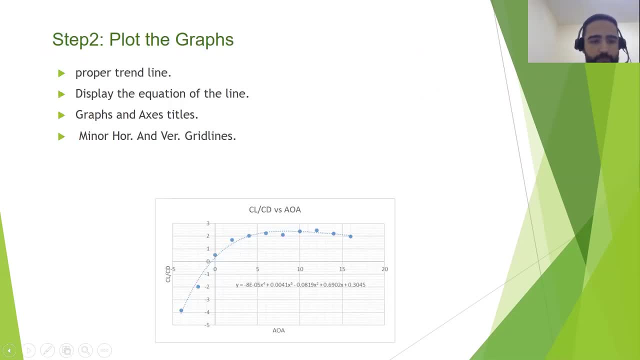 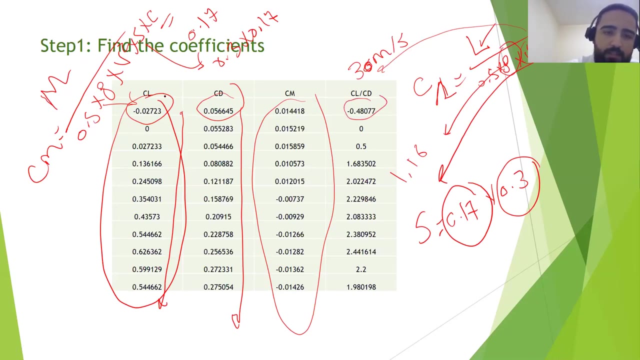 c, 0.17, s, 0.3 multiplied by 0.17. okay, after that here, divide this value, cl divided by cd, and put it here and in the similar way you can find the other, you can find other cells value. okay, now we have cl, cd, cm, cl over cd. 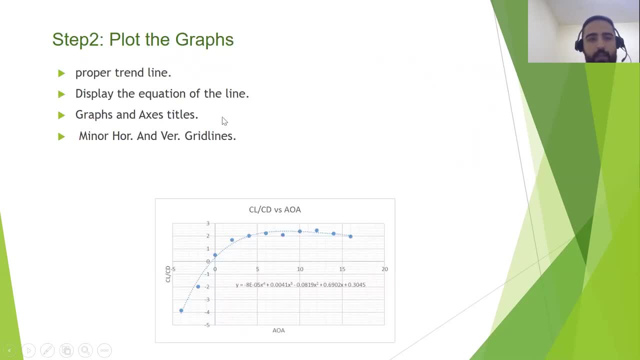 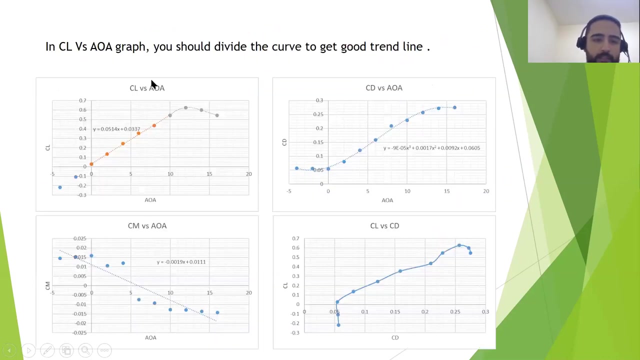 columns. what else now? step number two: plot the graphs. we will plot cl over cd versus angle of attack. we will plot cl versus alpha, cd versus alpha, cl versus cd, cm versus angle of attack. but while you are plotting these plots or these graphs, you should take in your consideration: 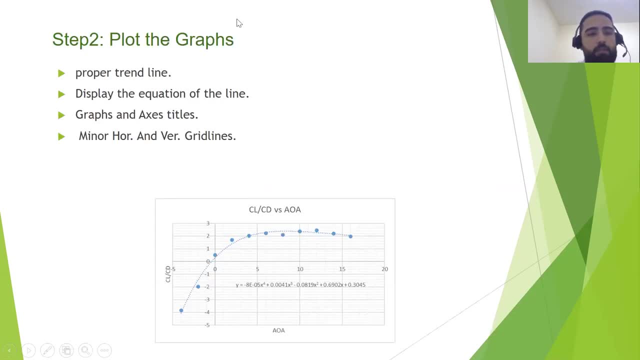 the following instructions. first of all, you should use a proper trendline, the dashed line. look at this. we have blue dashed line. this is the trendline, so you should use the proper trendline. if it's linear exponential polynomial, for example, in cl over c, d we will use exponential, for Plaid comes for CL because it's normal exponential phenomenal. exponential polynomial for Tucson multiplied by c for cm. but something for Randol and Al relaxing. and that was it and we will come to the next slide. next slide shows a construction system business map. as we talk about what is conservation patt and 1A in this science method, off machine. 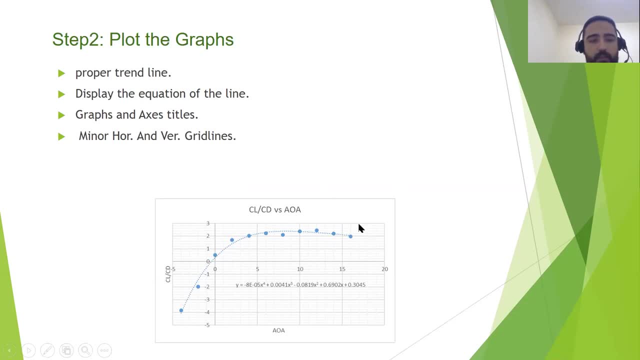 now, so i put different elements into it that are now know and use as two Beast terms of note: potential trend line. after that you have to display the equation of this line on the graph. this is the equation. put the axis titles and insert. change the setting of the picture from this button. 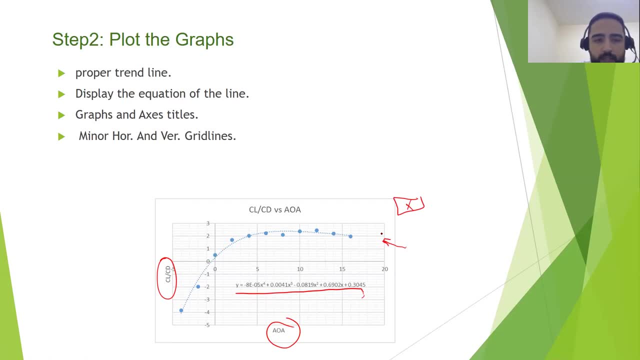 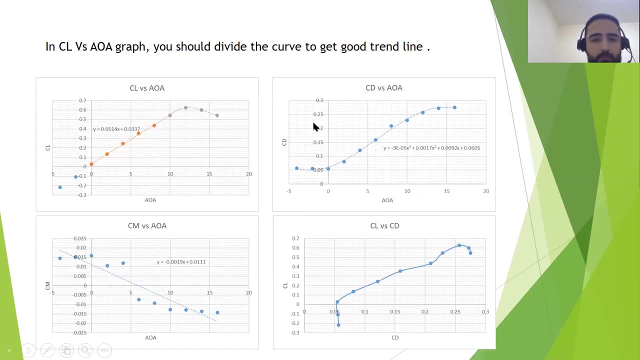 to show the minor horizontal and vertical grid lines. let us take a look here. this is for coefficient of drag and angle of attack and this is the equation. this is the axis titles and this is the title of the graph with. you can see here the minor vertical and the horizontal grids. 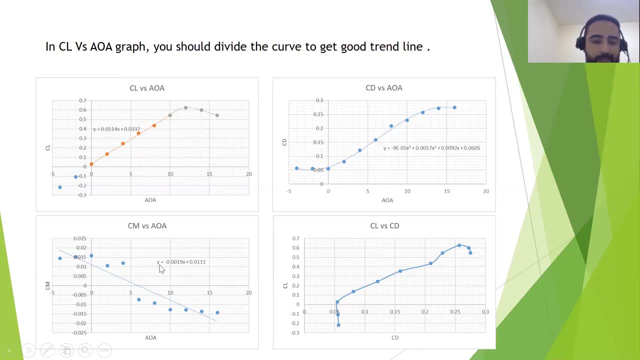 or and and grid lines in cm versus alpha. look at here, even if you have different points at different locations. but all of us knows that at low range of angle of attack, the relation between coefficient of moment and the angle of attack is linear. so put linear and. 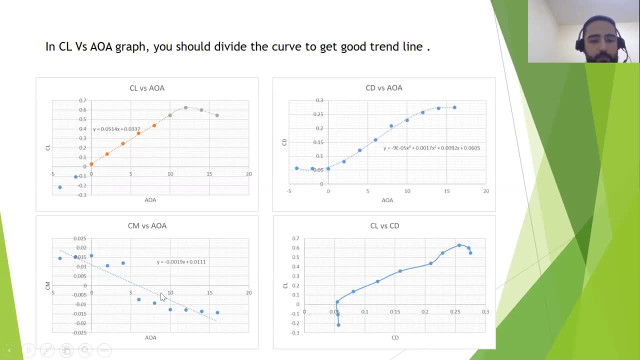 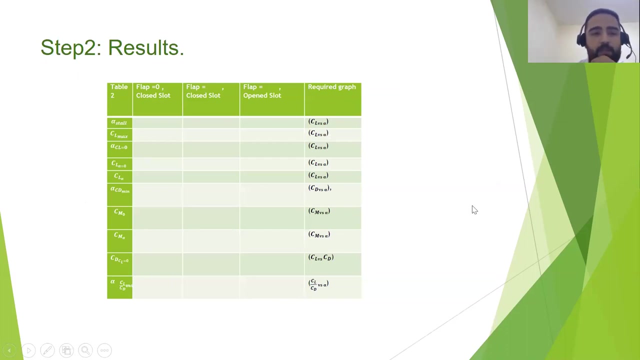 nonlinear. here two points: 2, 2, 8, 4, 8, 9, 10 interval for the linear relation and the second interval for the polynomial relation. why, to make a proper fit and to find exact number of the slope for this curve after plotting the diagrams, you should fill in this table. this is the 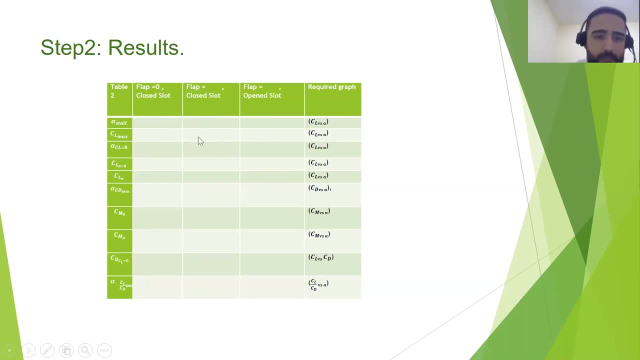 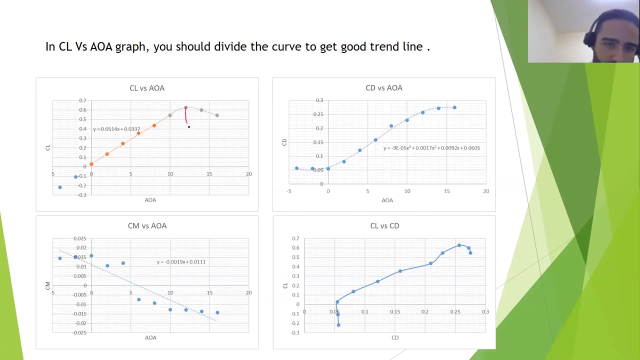 table of the results. for example, we need alpha stall for the first case, the second case and the third case. from which graph shall we measure this values? we have to go there. go to CL versus alpha, for example this one. where is the alpha stall here? just make a drop down which is equal to 12, for example, 12 degree, the. 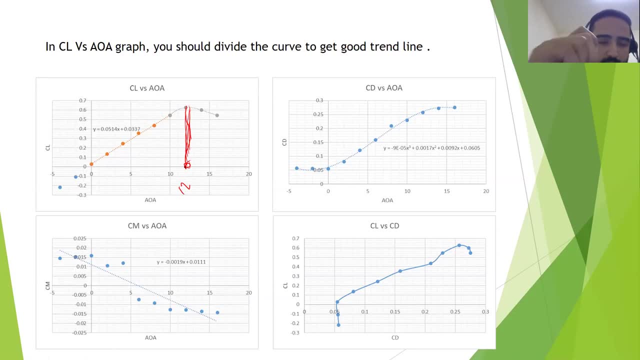 stall angle here is 12 degree, but here we just mentioned that. here we have a fake example, but in the experiment you have three cases here. one, two, three- this is for closed flap and the closed slot. this for closed slot and 23 degree of a flat, and the third cares for open slot and 23 degree. 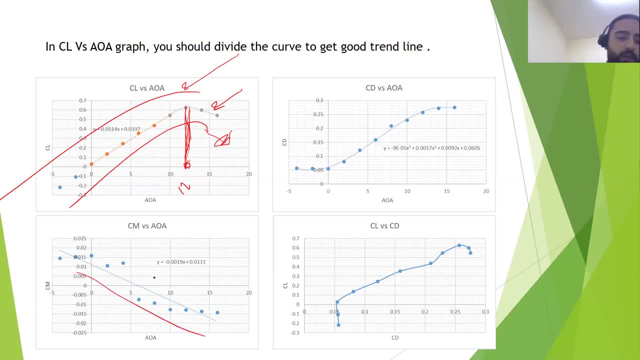 of flap angle, and here also we have a three, here we have three also and here we have three cares. each figure has three cares for three cases. from this figure we can measure the slope from which the curve will be measured to the angle, and here the stall angle, and here the stall angle, and we can fill in the. 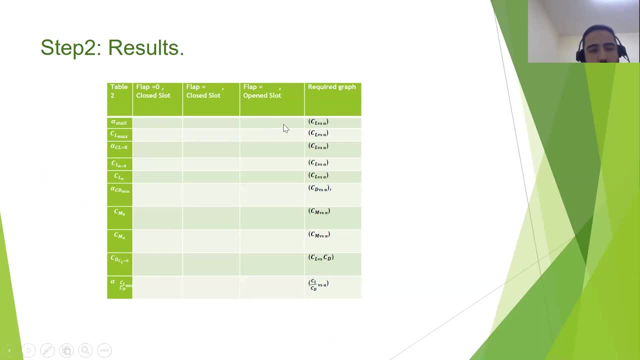 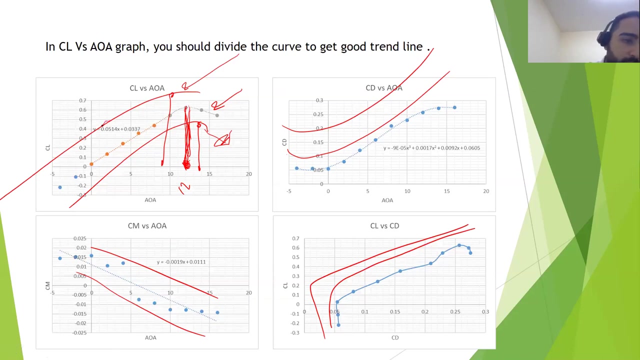 first row of the table. for the second row, we can measure the CL max from this, from the cell from the same paragraph: alpha at CL equals 0. CL at alpha equals 0 CL. alpha- this is the slope, for example. this is CL alpha or the slope. 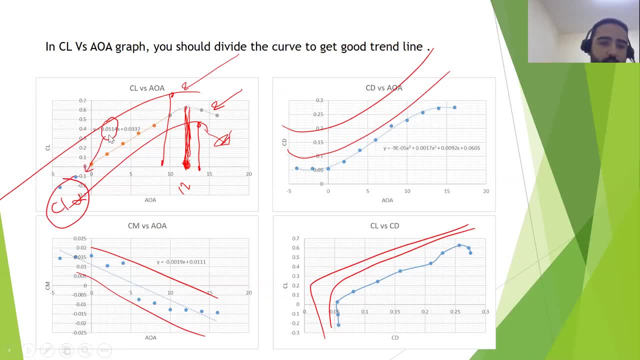 as we mentioned before, the value beside the X means the slope in the line equation. this the intersection with alpha, as we mentioned before, the intersection with y-axis. that's mean when X equals 0, so this is CL at alpha equals 0, which is equal to 0.0337. and do a similar thing to: 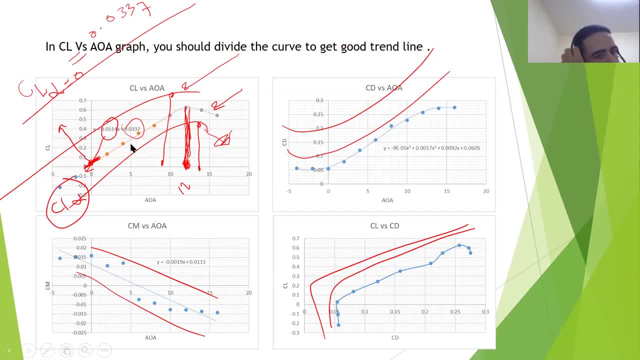 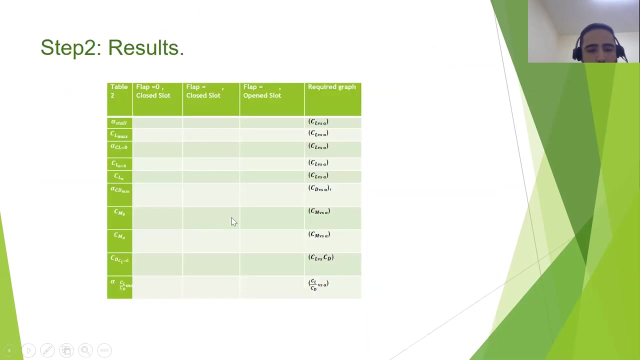 other two curves, this one okay. so here you need alpha, stall, CL max, the slope of the of the linear region, the intersection with y-axis and the intersection with x-axis. you, you, you properties. you need to reduce the slope, and anotherial program, which is KM alpha. 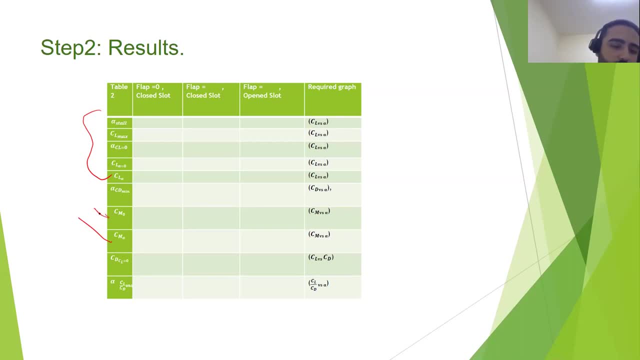 so KM on this line is the slope of cже000 in the hippocampus advantage and you you can find the graph what you are going to look at to measure these values. I hope you can find all of these tables from three graphs. each graph has three.